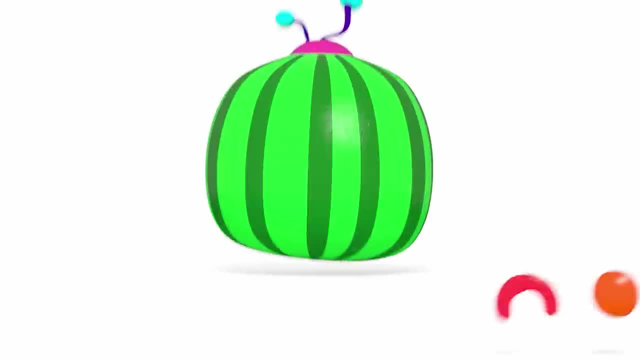 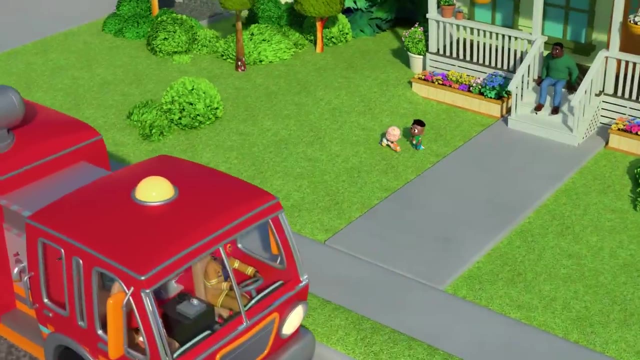 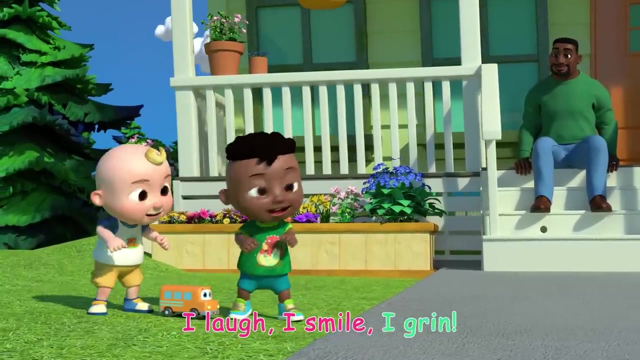 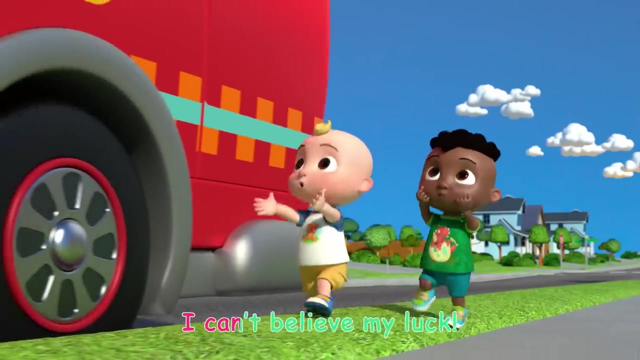 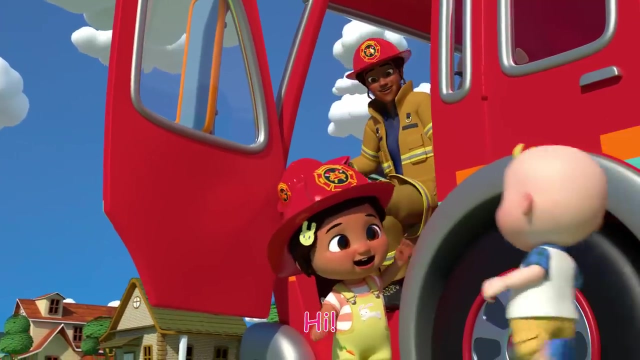 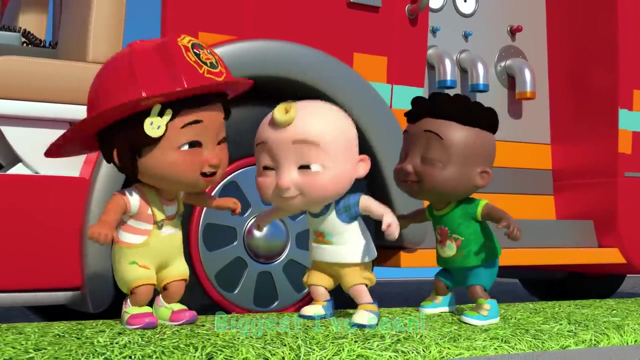 Cocomelon: Wow, A fire engine. I laugh, I smile, I grin. It's a real-life fire engine. I can't believe my love. It's a real-life fire truck Wheels- so big, big, big, Biggest I've seen. 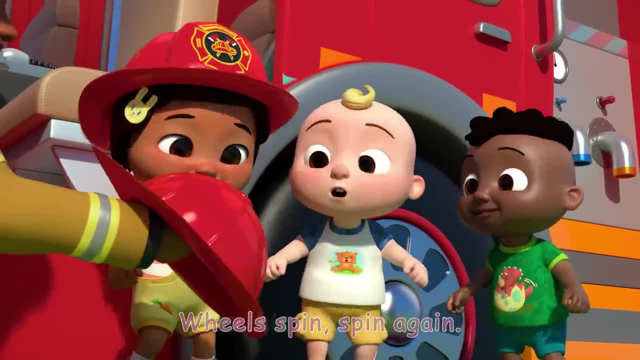 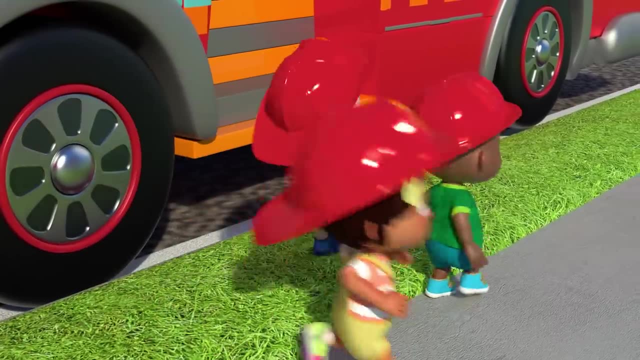 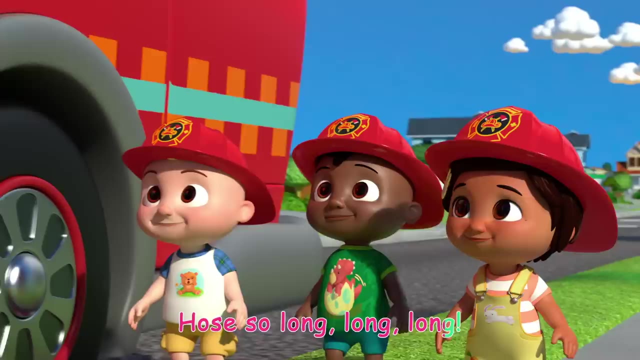 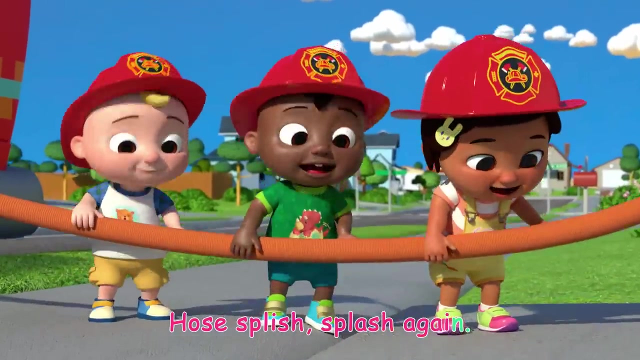 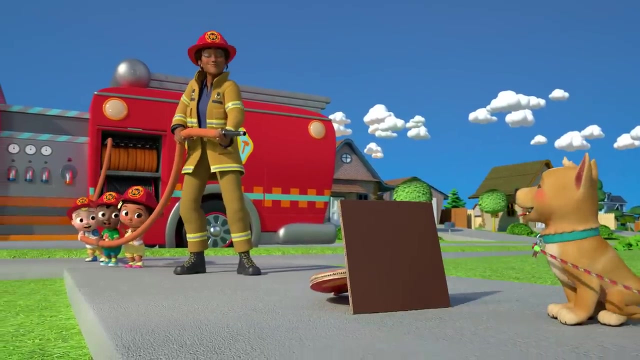 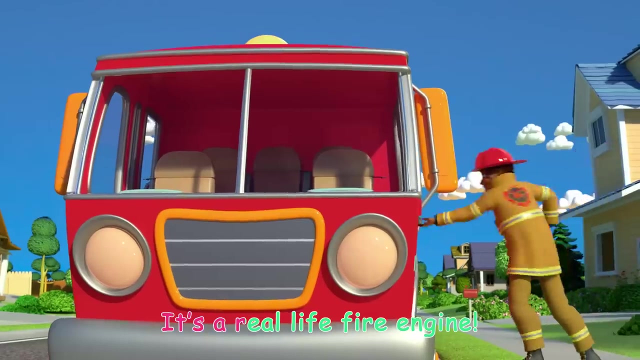 Wheels spin, spin again On this fire engine. Hey, Hose, so long, long, long Longest I've seen Hose splish, splash again On this fire engine. I laugh, I smile, I grin. It's a real-life fire engine. 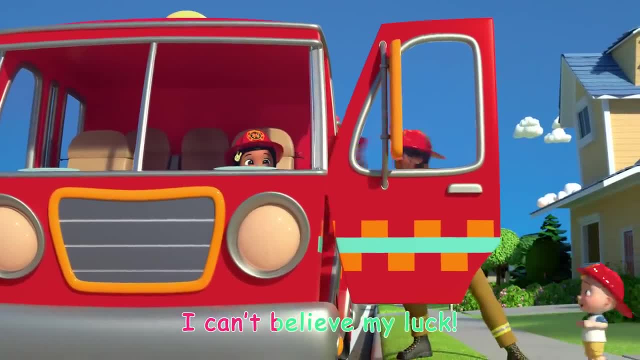 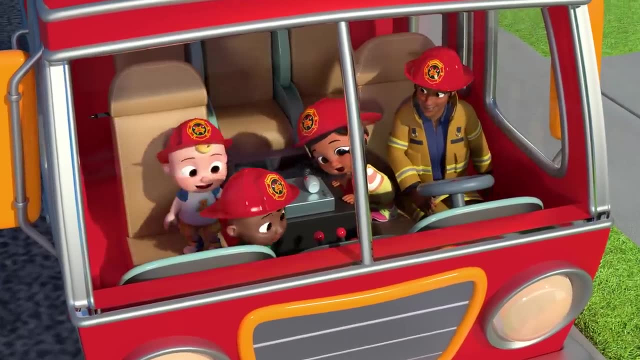 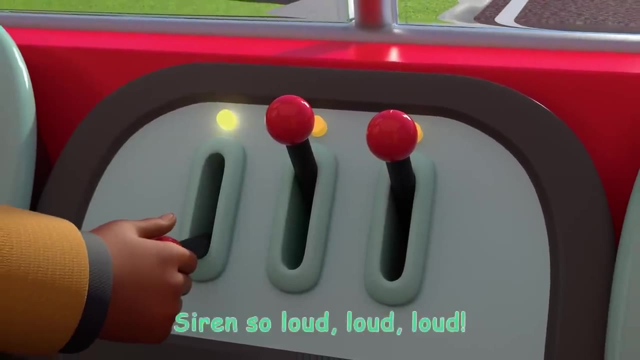 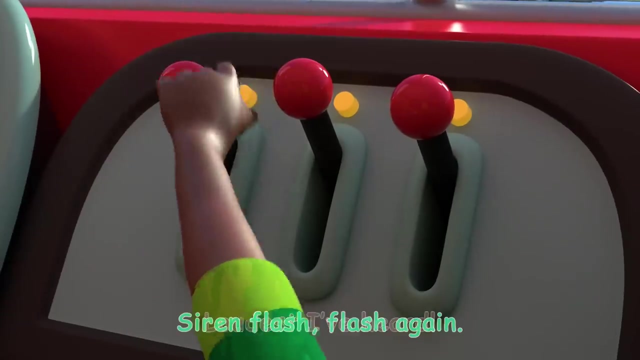 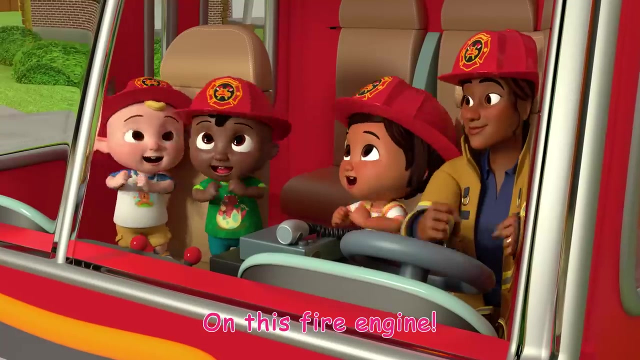 I can't believe my luck. It's a real-life fire truck, Sirens so loud, loud, loud, Loudest. I've heard Sirens flash flash again. Yeah, Yeah, Yeah Yeah. It's a real-life fire engine. 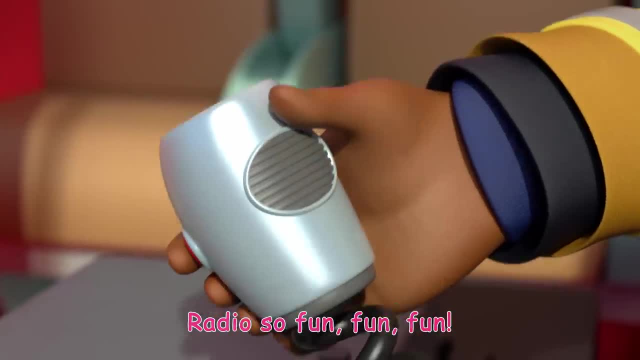 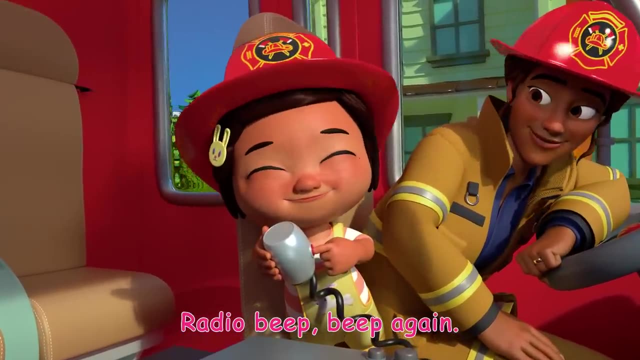 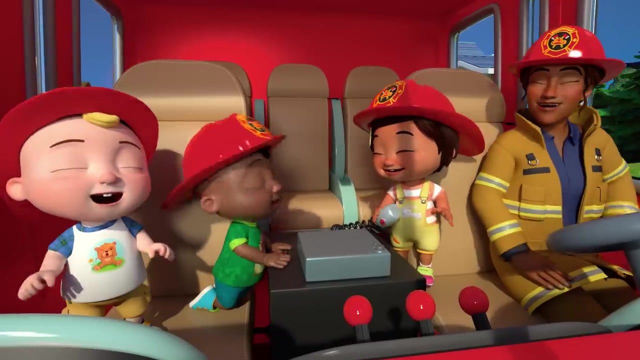 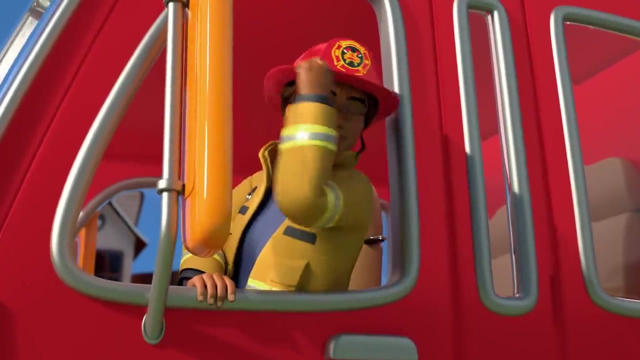 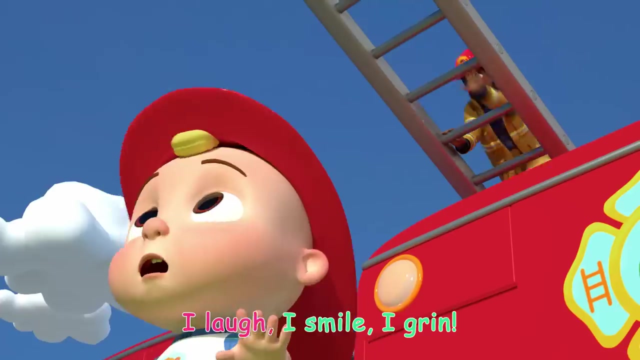 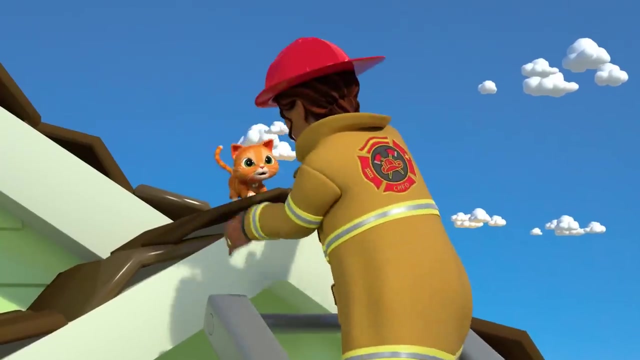